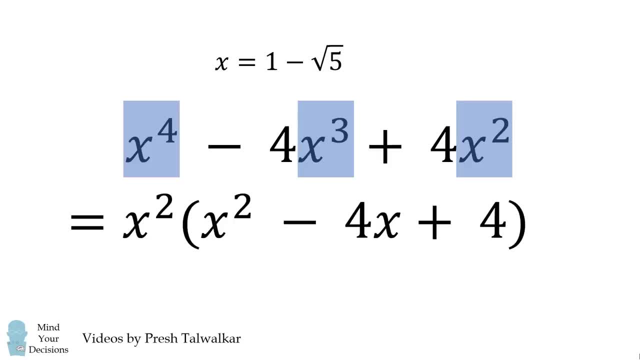 at these x terms, We can factor out x squared. Then we're left with a quadratic equation which we can further factor. This is equal to the quantity x minus 2 squared. We then further simplify by taking the exponent outside this grouping. Now let's substitute: x is equal to 1. 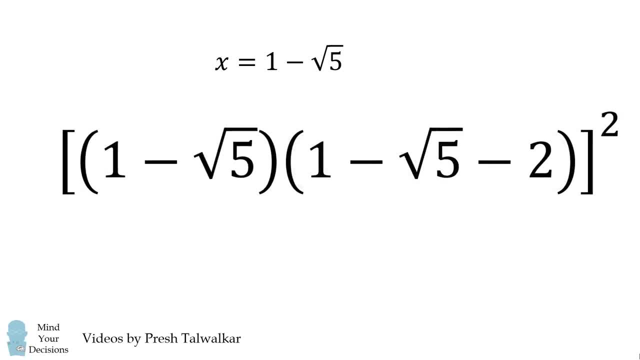 minus the square root of 5.. The second factor will simplify to be negative: square root of 5 minus 1.. We'll now flip the terms in the first factor. The reason we're doing this is that we get a product of a sum and a difference which will be equal to a difference of squares. So this will be equal to 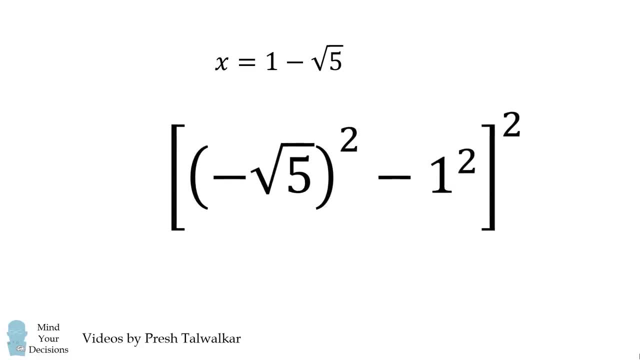 negative square root of 5 squared minus 1 squared. The first term will simplify to be 5, and then we have 5 minus 1, which is equal to 4.. 4 squared is then equal to 16, and that's our answer. 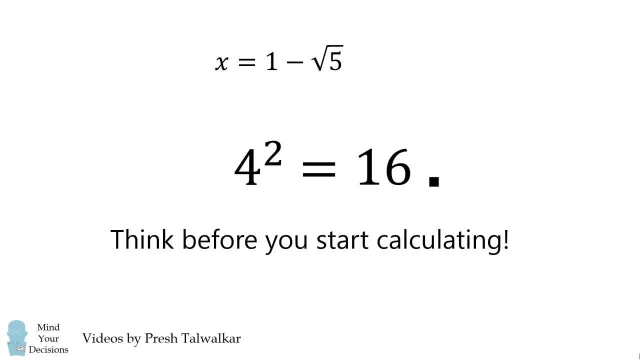 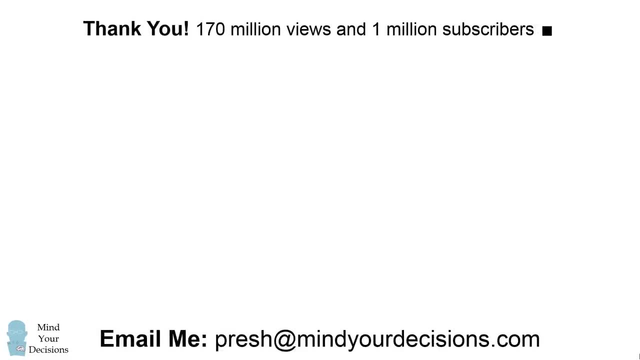 The lesson is that it sometimes helps to think. Think before you start calculating. Thanks for watching and for making Mind Your Decisions. one of the best channels on YouTube. Thanks for watching and thanks for your support. 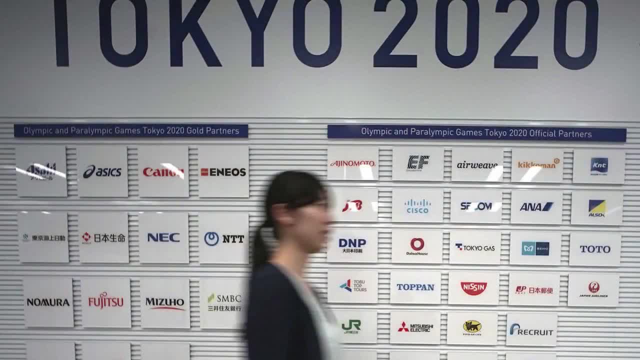 Seoul, South Korea, AP. the Winter Olympics coming to South Korea in February offer an example of the Olympian efforts often required to meet corporate sponsorship goals. Tokyo tells a different story. the coffers are already overflowing for the 2020 Summer Games. It's a tale of two cities in two Olympics: winter and summer. 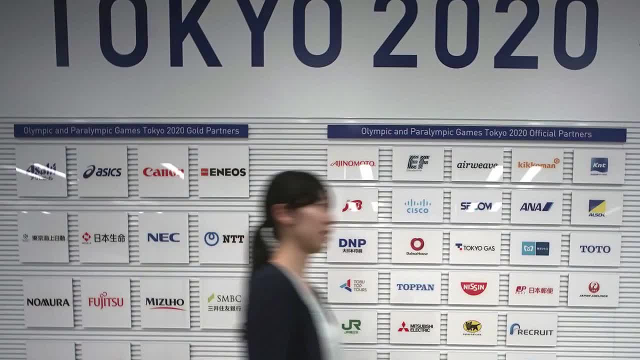 Pyeongchang is a little-known destination in one of South Korea's poorest provinces. It is the little town that could bidding twice unsuccessfully for the Winter Olympics, before winning on its third try. A final push enabled it to reach its sponsorship target of $940 billion in September, with just five months to go. Tokyo is an established global capital and the Summer Games usually generate more excitement And more money. Organizers have raised 300 billion yen- $2.7 billion- in sponsorship- twice any previous Olympics. International Olympic Committee Vice President John Coates describes it as a remarkable achievement. The divergent experiences of two Asian host cities illustrate the challenges that smaller bidders face, as well as South Korea's dependence on the big family-owned companies that dominate its economy. The big family-owned companies that dominate its economy. The big family-owned companies that dominate its economy.